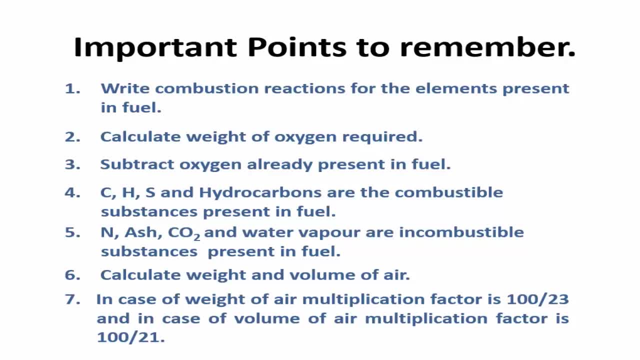 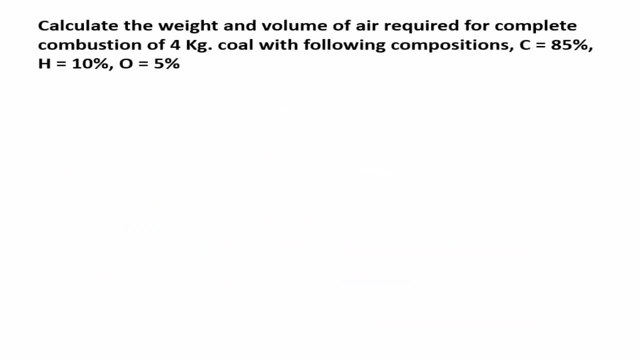 the multiplication factor is 100 upon 23.. When we have to calculate volume of air, the multiplication factor is 100 upon 21.. Let us see the first numerical Calculate the weight and volume of air required for complete combustion of fuel. So drop the kelvin ratio into Fasc to find out the percentage of carbon. 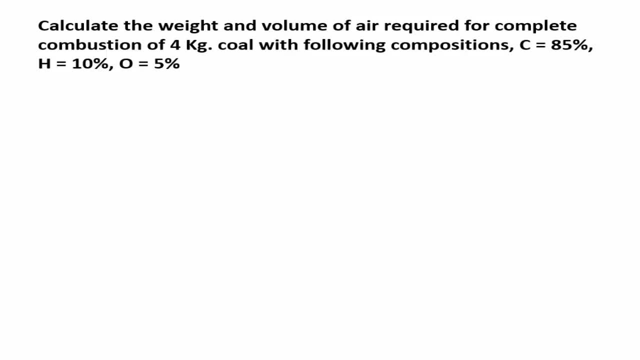 If it is 0.4 kg of coal with following compositions: Carbon 85%, hydrogen 10%, oxygen 5%. So, as I discussed earlier, we have to write the combustible reactions first. The first one is carbon. The combustible product of carbon is CO. So from the reaction we can: 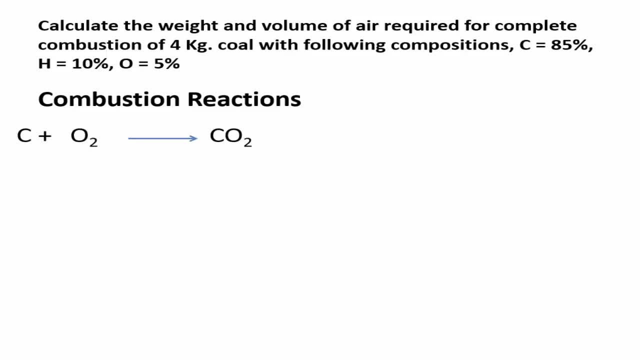 predict, for 1 mole of carbon, 2 moles of oxygen will be required for the combustion weight. we can say that for 12 moles of carbon, 32 moles of oxygen will be required to produce 44 moles of carbon dioxide. so for these elements we have to. 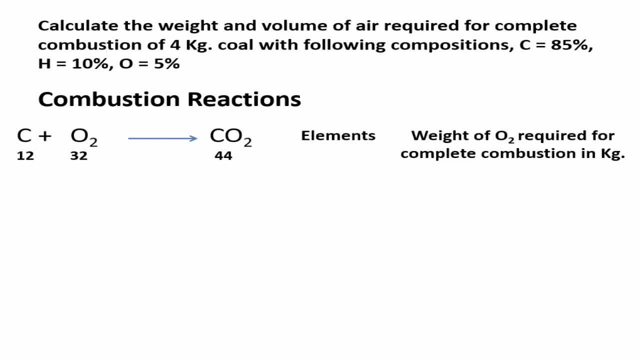 calculate the weight of oxygen required for the combustion. as in the numerical, 85% of carbon is present, that is, 0.85 kilogram of carbon is present. so we will multiply, using the equation, 0.85 into 32 by 12, so total 2.26 kilogram of oxygen. 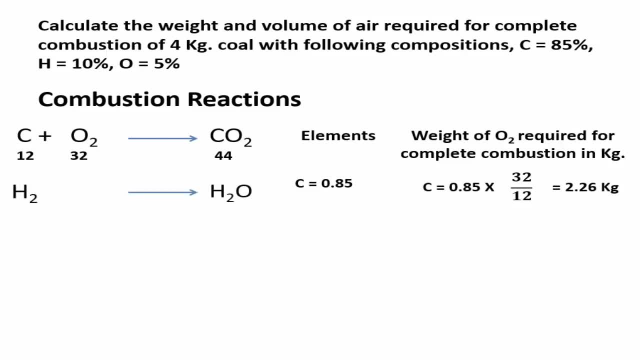 is required for the combustion of carbon. similarly, for the hydrogen, half mole of oxygen will be required, and and for 2 moles of hydrogen 16 moles of oxygen will be required. so weight of oxygen required will be calculated as 0.8 kilogram. we. 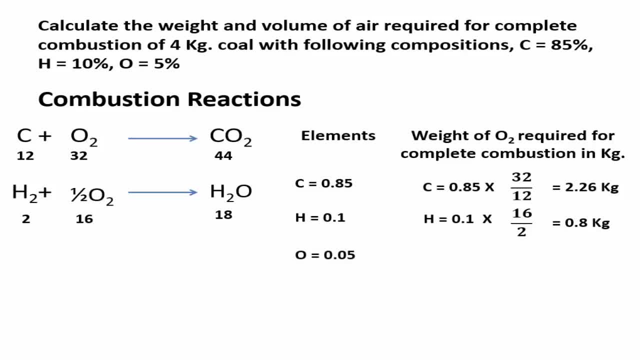 have to remember that 5% oxygen is already present in the fuel. you have to remember that 5% oxygen is already present in the fuel. you have to remember that 5% oxygen is already present in the fuel. you have to remember the total amount required for oxygen retyping. we need to subtract it from the 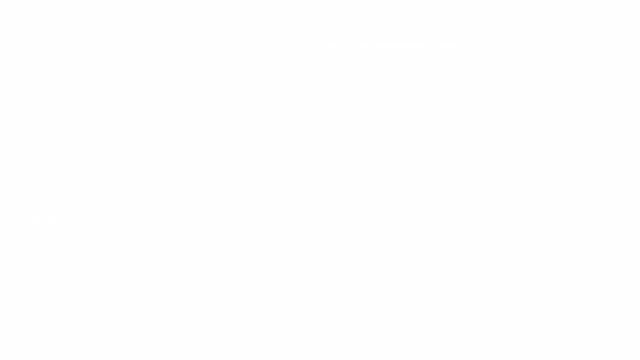 total oxygen. the total oxygen calculated is 3.06 kilogram. we removed further, we know that weight of oxygen required will be weight of oxygen needed minus weight of oxygen present. so 3.06 was the total oxygen which was present. so we have subtracted 0.05. so net oxygen required will be 3.01 kilogram. from this we can 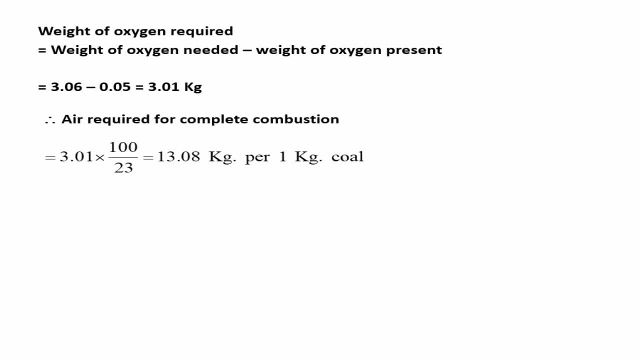 calculate the air required, 23% of oxygen is present by weight. We will multiply it by 100 upon 23.. So total 13.08 kilogram per 1 kilogram of coal is the amount of oxygen required for the combustion of coal. 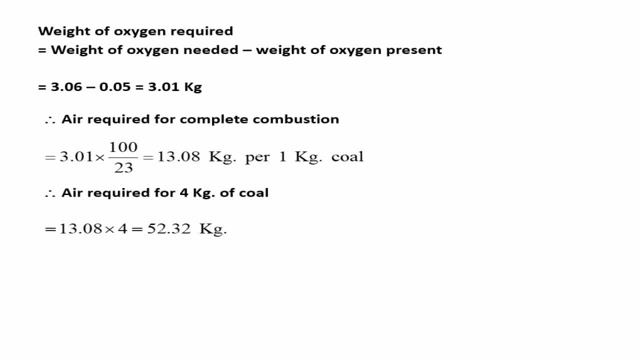 Therefore, for 4 kilogram of coal, the amount will be 52.32 kilograms. Now we will calculate volume of air required. There is one equation that we have to remember, that is: 28.94 kilogram of air is equal to 22.4 liters of volume of air at normal temperature pressure. Using this equation, 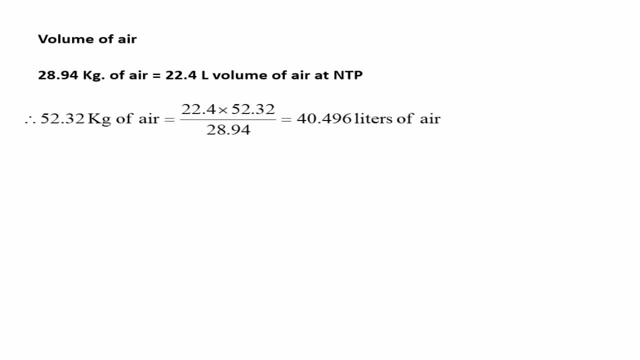 we can calculate it as 40.496 liters. So our final answers are, by weight, 52.32 kilogram of air required and by volume. We move to the second type of problem. A gaseous fuel has following composition by volume: Methane 25% carbon monoxide, 10% hydrogen. 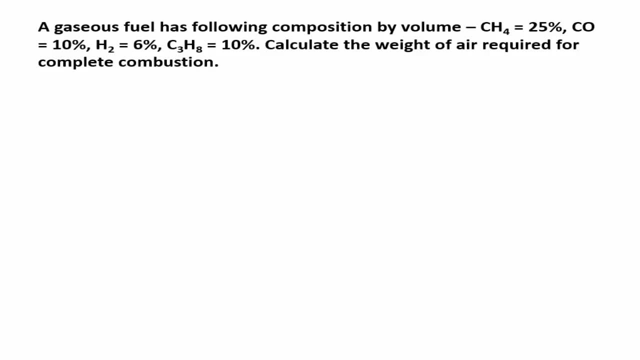 6%, propane: 10%. Calculate the weight of air required for complete combustion. Now you need to remember that the composition is by volume. So first we will have to calculate by volume and then we need to calculate by weight. If the composition was given by weight, 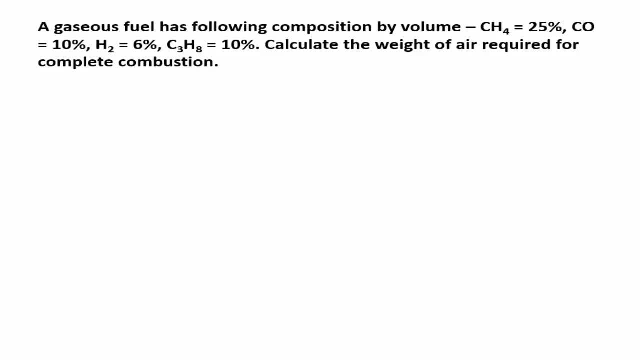 then we would have calculated by weight first, and from that we would have calculated by volume. So first we have to write the combustion reactions. First is methane. All hydrocarbon on combustion gives only two products. First is CO2 and second is H2O, As there is only one carbon. 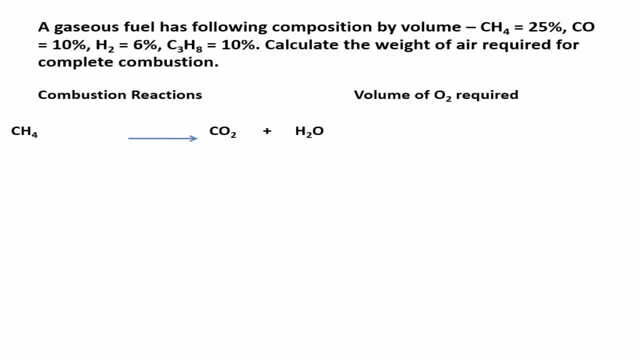 one CO2 will be produced and four hydrogens. that means two molecules of water will be produced. So we will require two moles of oxygens. That means for one volume of methane two volumes of oxygen will be required for the combustion. So we will calculate volume of O2 required as 0.5. 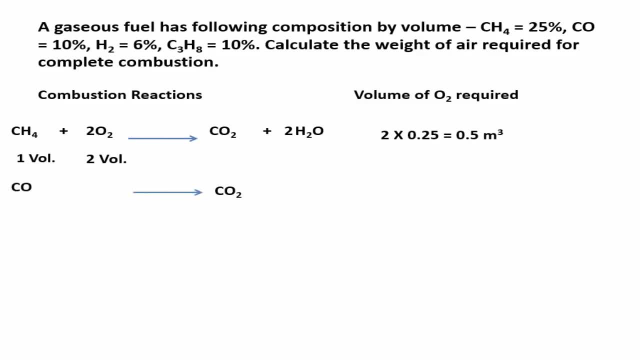 meter cube. In the similar way, we will calculate the volume of oxygen required for the combustion. In the similar fashion, for carbon monoxide, half volume of oxygen will be required and the total volume will be required as calculated: 0.05 meter cube. Third is hydrogen. For two volumes of hydrogen, 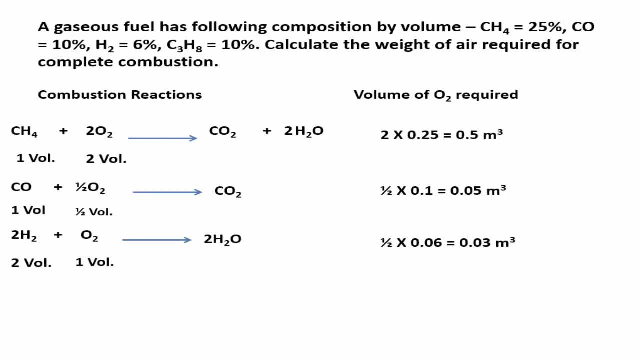 one volume of oxygen will be required, and the volume required for oxygen total will be 0.03 meter cube. Fourth is propane. Three carbons are present, So three moles of CO2, and total eight hydrogens are present, So four moles of H2O. 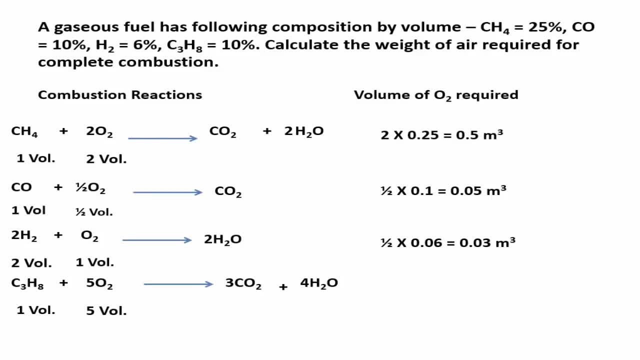 Thus, for one volume of methane, five volumes of oxygen are required. So total oxygen is 0.5 meter cube. So for all these elements the total oxygen required is 1.08 meter cube. Now there is no. 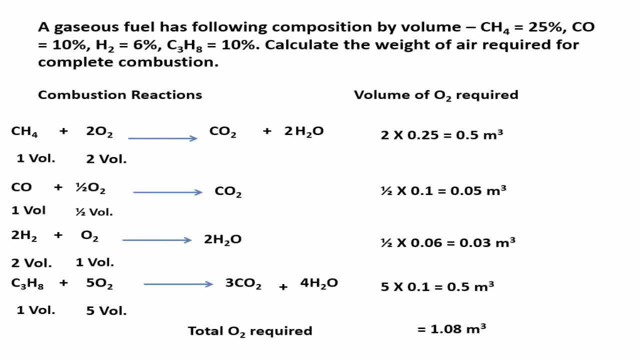 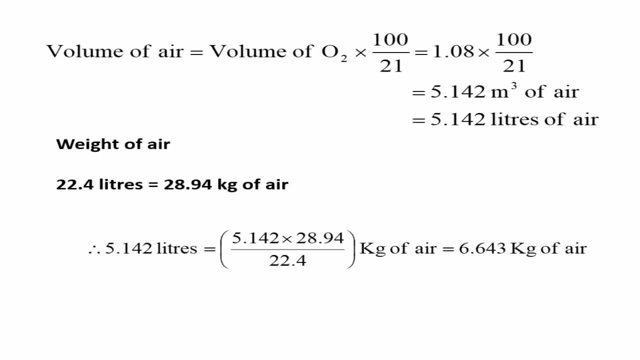 oxygen present in the fuel, So no need to subtract any oxygen. So we will calculate directly the volume of air. While calculating we have to multiply it by 100 by 21, because by volume 21 percent of oxygen is present. 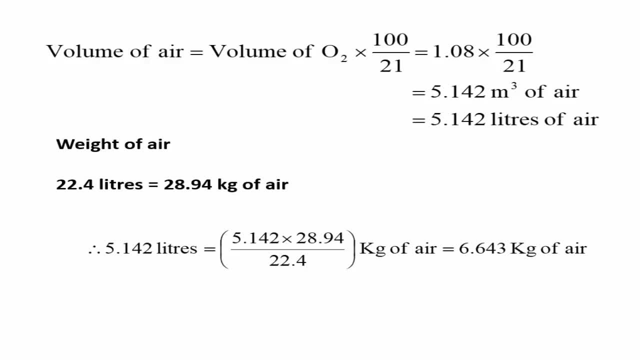 calculated as 5.142 meter cube or liters of air. So from this, as in the earlier case, we have calculated from the equation: 22.4 liters is equal to 28.94 kg of air, So 6.643 kg of air is required. 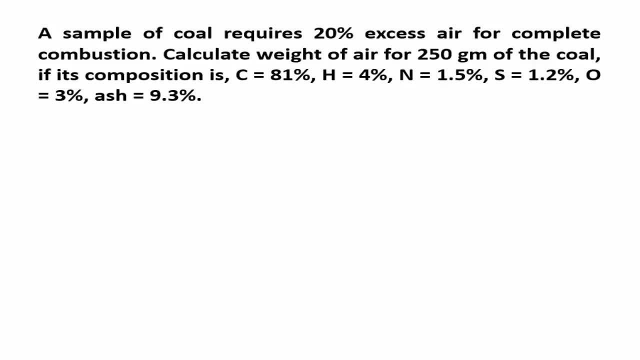 Now we move to the third type. In the third type we can see that a sample of coal require 20% excess of air for complete combustion. That means, compared to normal coal or normal fuel, 20% excess air is required. Calculate the weight of air for 250 gram of coal if its composition is: 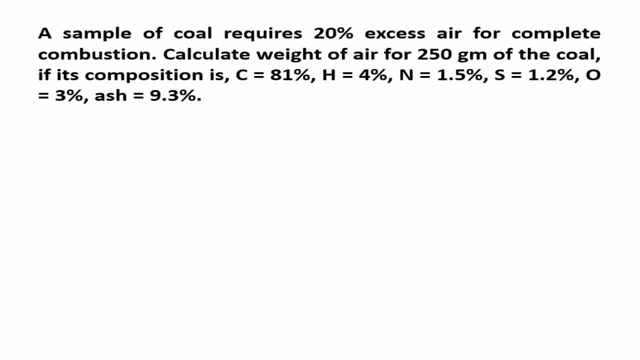 81% carbon, 4% hydrogen, 1.5% nitrogen, 1.2% sulfur, 3% oxygen and 9.3% ash. Remember that if nothing is given to the coal, then the coal will not be given to the coal. So 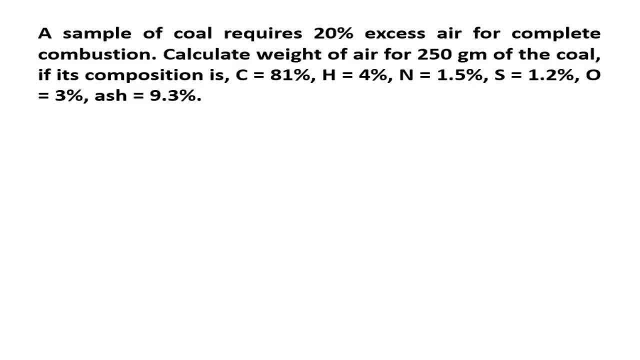 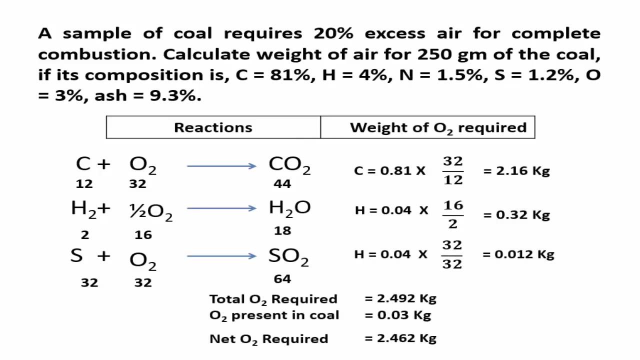 we have to consider. the composition is given by weight. So first we have to write the reactions and the weight of oxygen required. As in the earlier cases, we will calculate first the weight of O2 required for all those elements which are combustible. So total oxygen required is 2.492,. 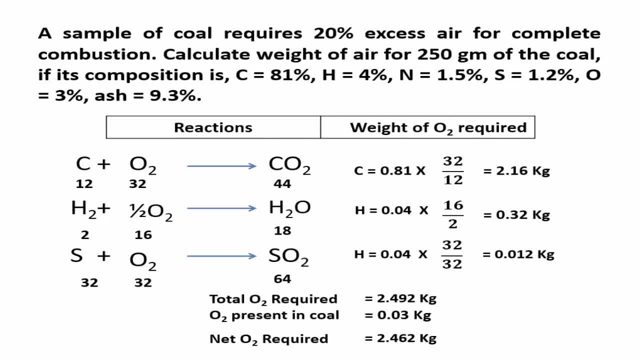 oxygen present is 3%, We will subtract it and net oxygen required is 2.462 kilograms. Now we move further, Weight of air required will be 1.5 kg of oxygen. So we have to write the reactions and the weight of oxygen required.